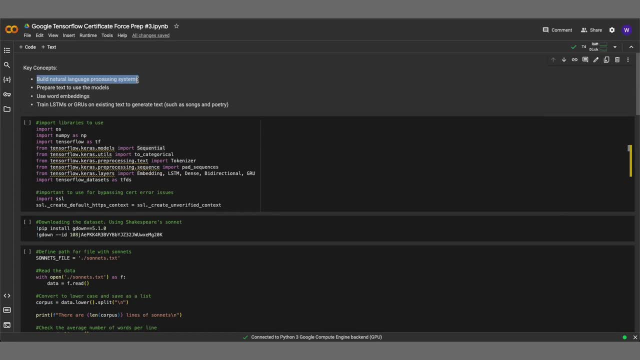 They are To build natural language processing models, Prepare text to use for models, Use word embeddings And, lastly, to train LSTMs or GRUs on existing text to generate text such as songs or poetry. As usual, let's import the libraries that we will be using today. You may notice a few new methods. 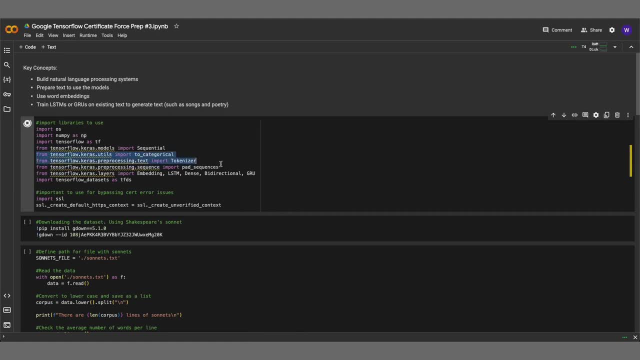 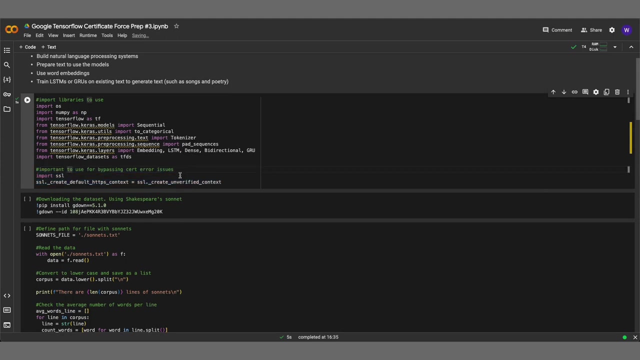 such as decategorical tokenizer, pad sequences and embedding. These are specific to natural language processing and we will be using them in our code later. Lastly, we will import SSL as well to resolve any certificate issues. if you are running this code from the computer After the libraries are downloaded, we will have to download the. 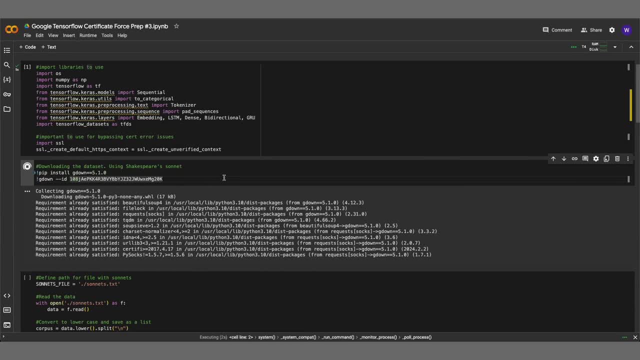 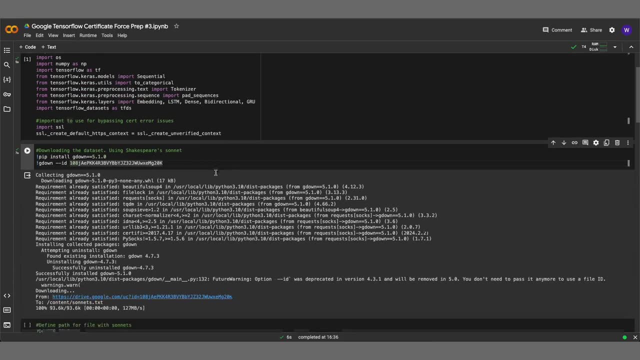 dataset as well. We will be using Shakespeare's Sonnet as our dataset and we will train the model on it to predict words and to create its own Sonnet as well. We will now inspect the file. We will read the saved text file and will then connect. If this epose is recommended in question, I will 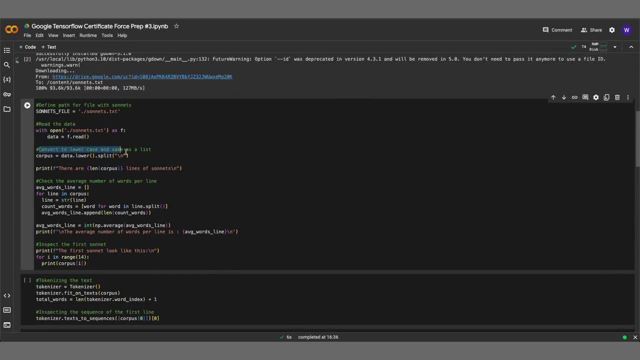 perform the process following the script and carries this from that file through the software Then, and convert all the letters to lowercase and split them by lines. we can print to see the number of lines in the sonnet database and to check the average number of words per line. we can also 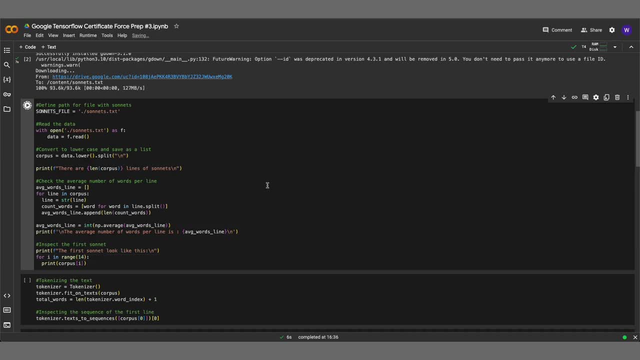 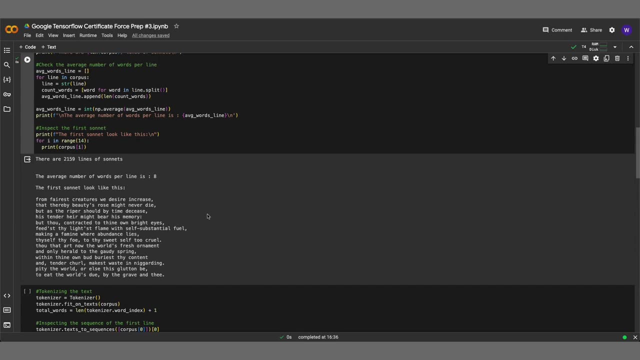 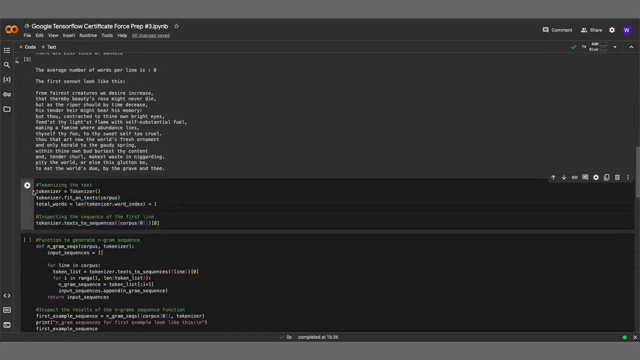 print to see how the first sonnet looks like. as we can see, the english they use is not modern english and it's shakespearean english. now we will tokenize the text, we will fit the text to the corpus, which will assign a number to each word in the database, and we will increment the total number. 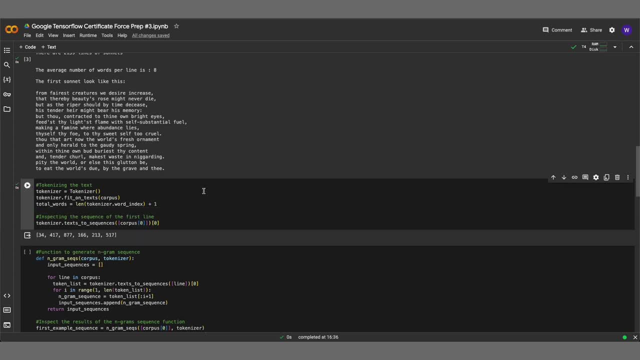 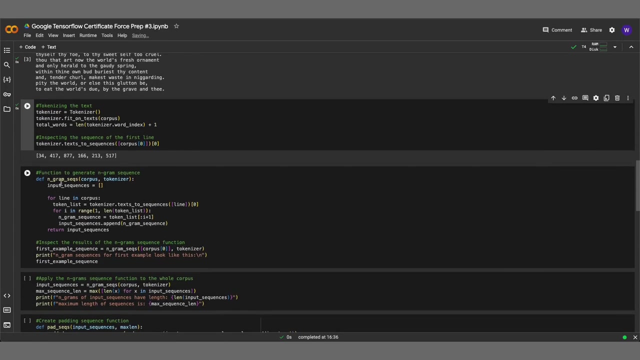 of words in the lexicon by one, as the starting number of the word index is zero and not one, we can inspect the sequence of the first line as well, as we can see from the results they have been converted to a list of numbers. next we will create a function to generate engram sequences. 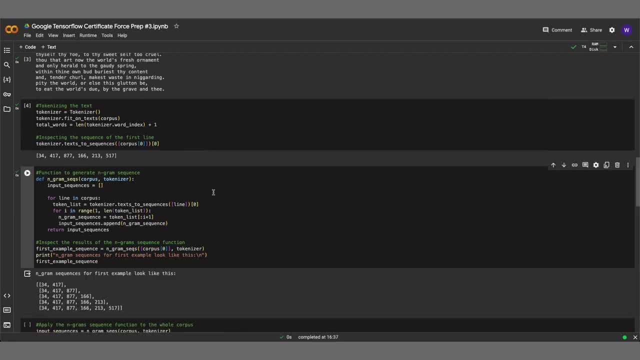 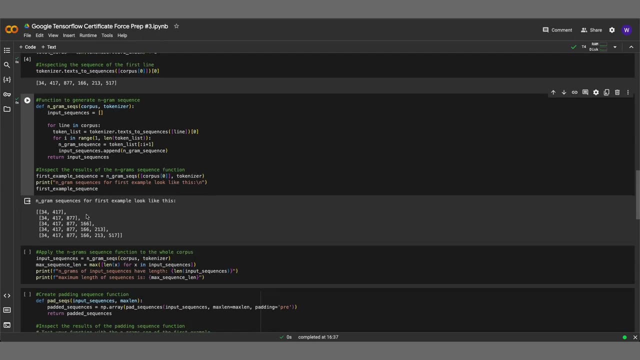 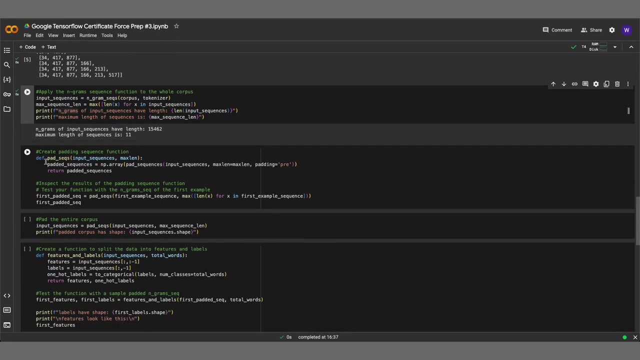 this will help in the model's understanding of context based on surrounding words. we can also print the results to visualize how the results look like. we will now apply the n-gram sequence on the corpus. next we will pad the n-gram sequences which we created earlier. this will help to normalize the 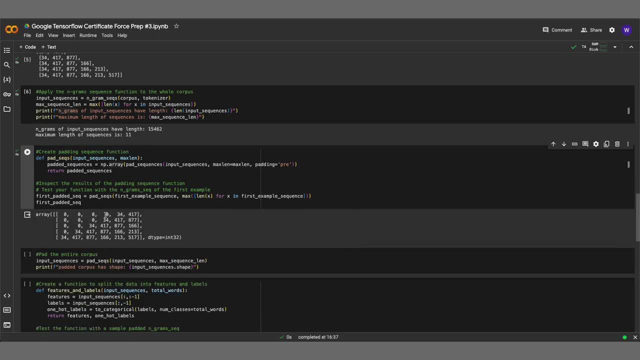 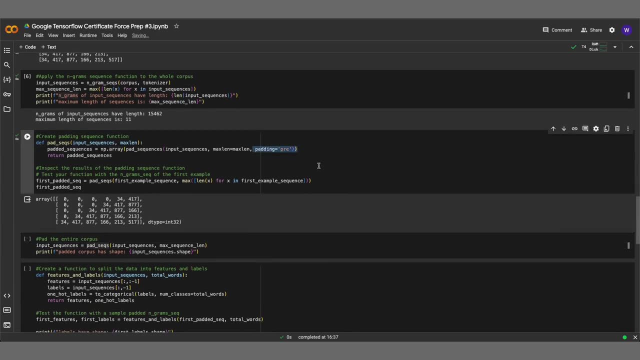 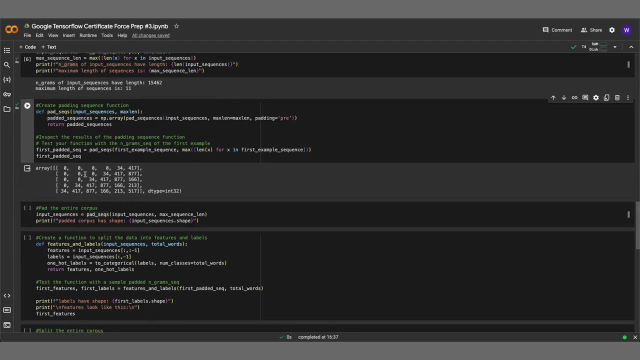 sequences such that they are all of the same length. we will apply the padding with pre so as to allow model prediction for the next word. if the padding is applied with post, the model will predict on the padding, which is not what we want. we can visualize it below here, once we have the 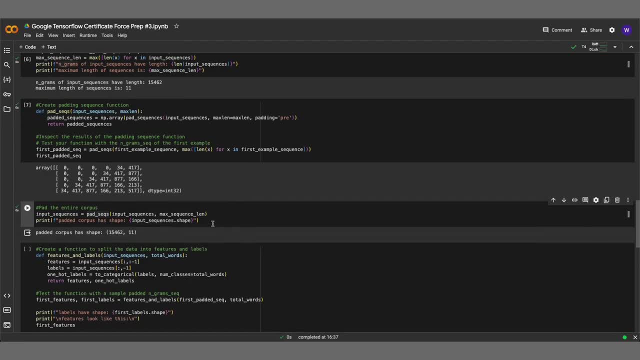 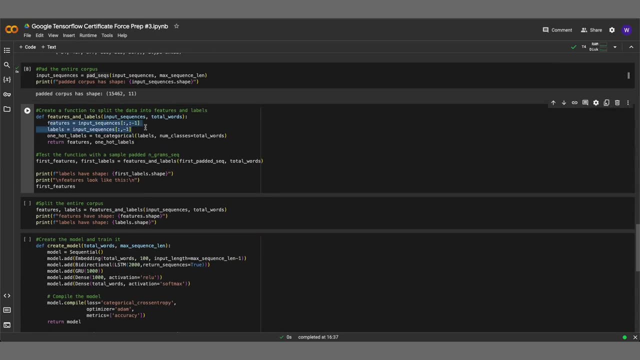 function ready, we can proceed to apply the padding to the entire corpus as well. next, we will create a function to split the corpus into features and labels. the features would be the padded n-gram sequences which we created previously, and the label would be the next word to continue in. 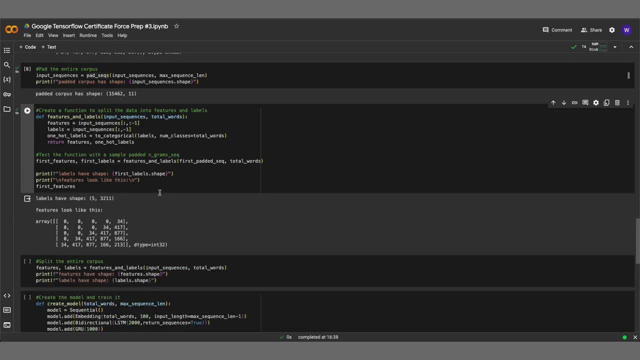 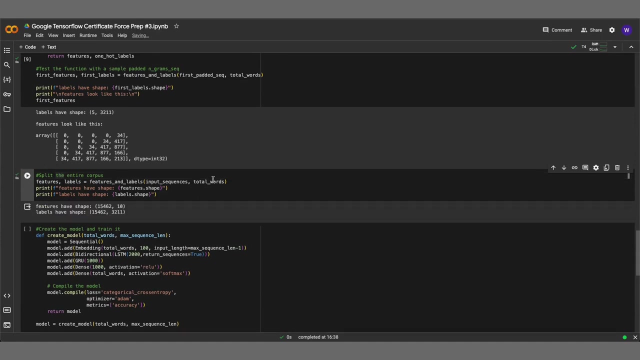 the sentence. we would apply one hot label encoding to the labels so that we can use entropy as our loss function in the model. later on We can print to inspect the shape of a sample label and to view the first features. The last step to pre-process data is then to apply the previous function to the corpus. 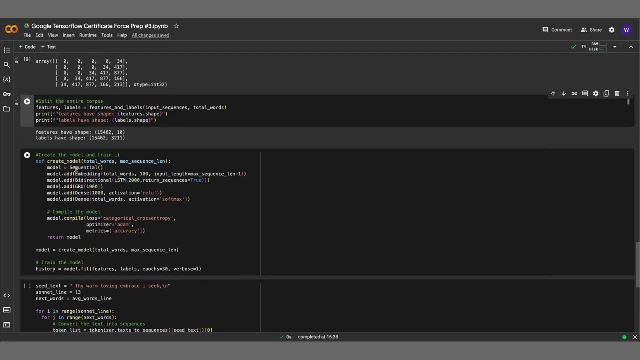 Now we will create the model. We will start with an embedding layer of the corpus and add a bidirectional LSTM layer followed by a GRU. We will then end off with two dense layers. The arguments passed into the compilation method are nothing too uncommon, and we can. 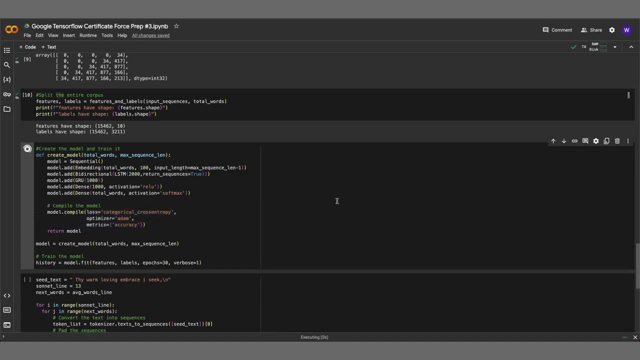 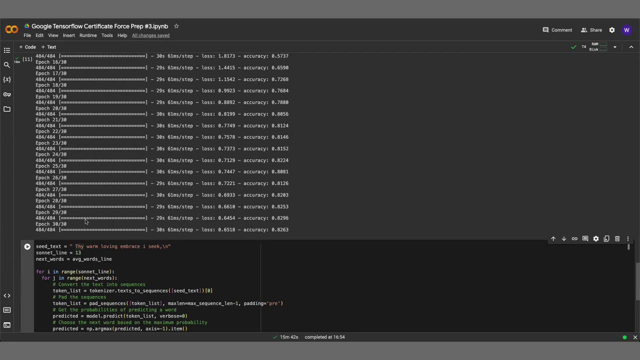 proceed to train the model. This is going to take some time, so I will skip the training here. That took quite a while, but the model has finally completed training At the end of 30 epochs. the accuracy is hovering around 82 to 83 percent. 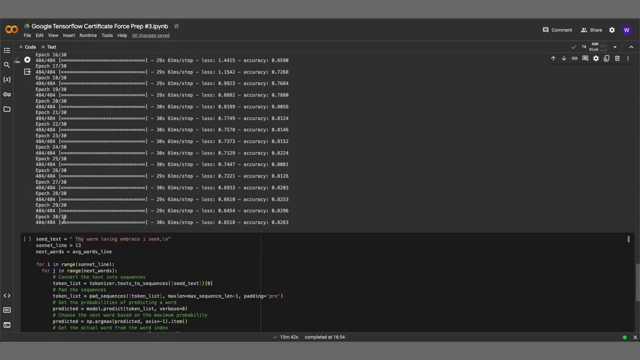 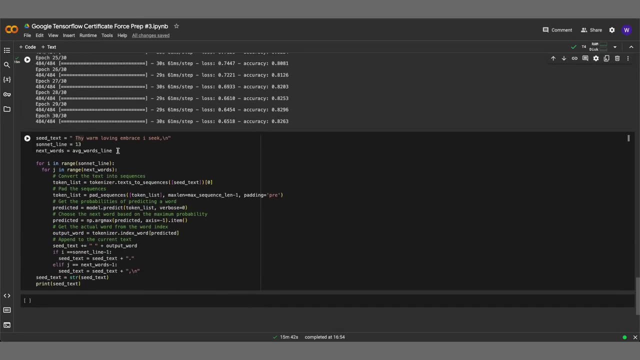 You can train it for longer if you like, but in the interest of time, let's continue. Now for the moment of truth. We will use the model to produce the model. We will use the model to predict texts or actually, more like, to create an entire sonnet. 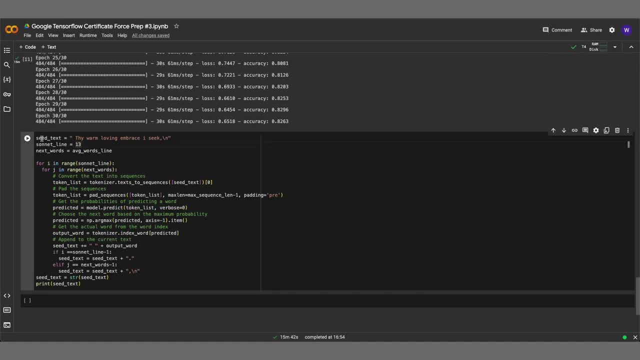 from a seed text. I will feed in a seed text line by warm, loving embrace. I seek and see what it comes up with. Based on what I have seen, a sonnet has 13 lines, so I set it here. Remember the average number of words from earlier. 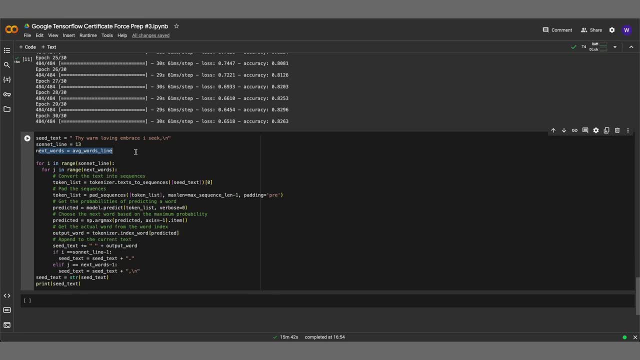 We will use it here to set the number of words per line of sonnet. Next I will iterate it over the range sonnet lines and for each word we will predict the next word with the highest number of words. This is the highest probability.